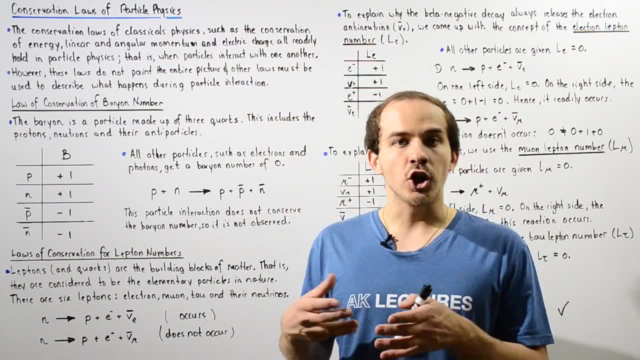 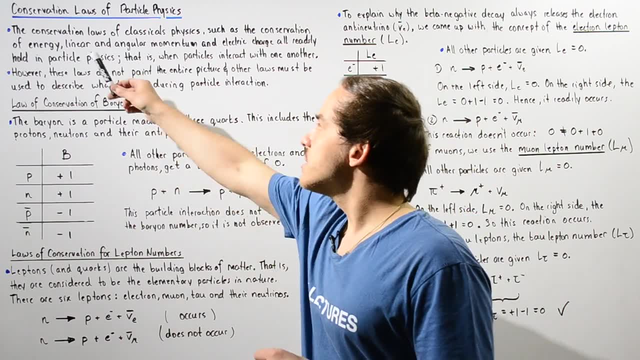 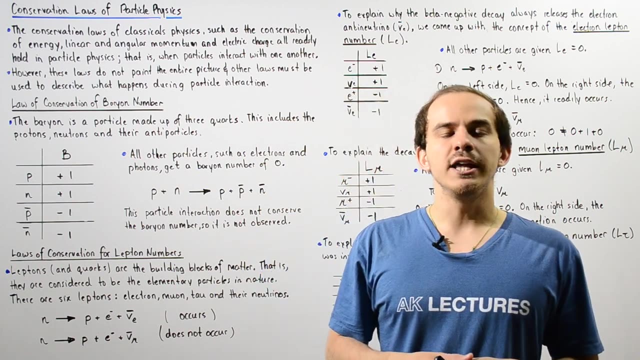 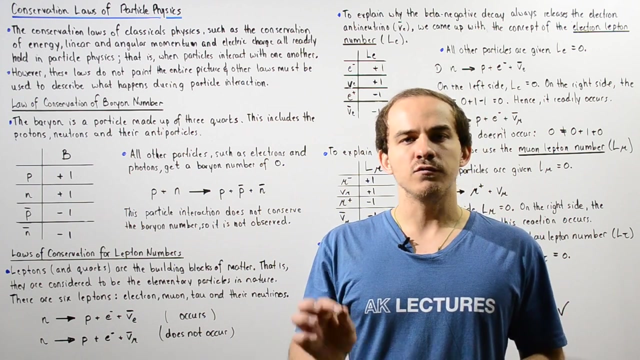 that the laws of conservation that we learned about in classical physics hold for these particle interactions. So the conservation laws of classical physics, such as the conservation of energy, the conservation of linear and angular momentum, as well as the conservation of electric charge, are all readily observed whenever we deal with our particle interactions. 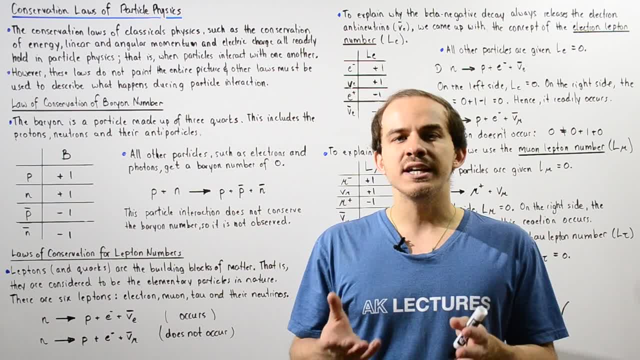 However, these four laws are not the only conservation laws that exist. Other laws exist when we deal with the conservation of energy. As you can see, this is the conservation law of quantum mechanics. When we deal with quantum mechanics, we deal with particle interactions. 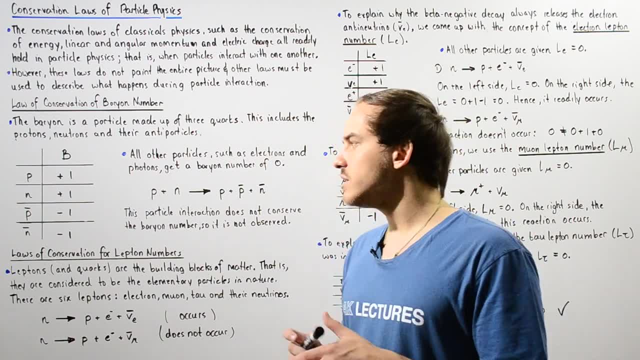 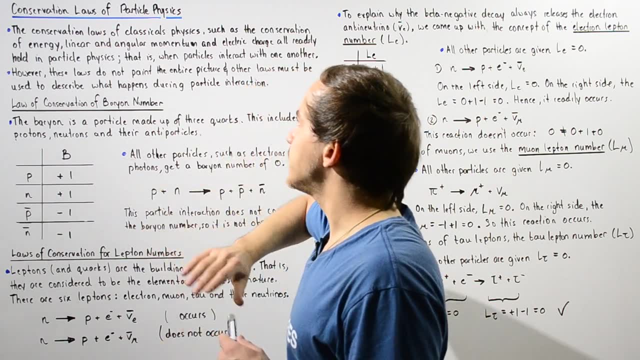 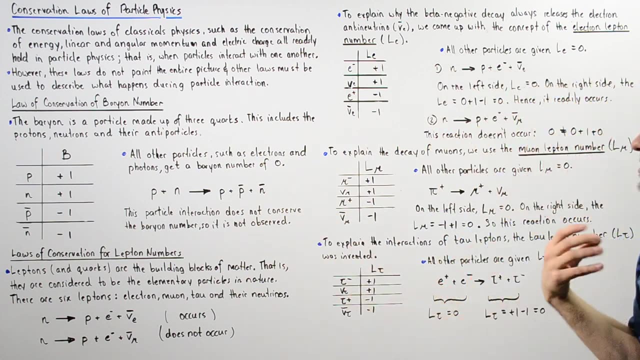 particle interactions, and those laws are the laws that we're going to discuss in this lecture. So, once again, these four laws that come from classical physics do not paint the entire picture of how particles interact in the subatomic world, and other laws must be used to describe what 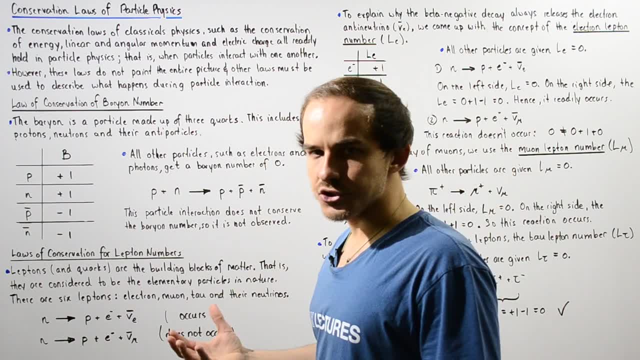 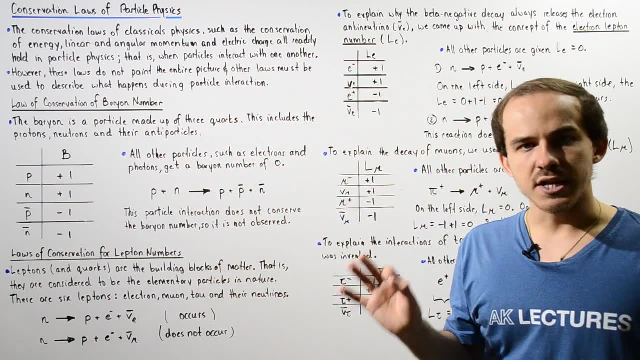 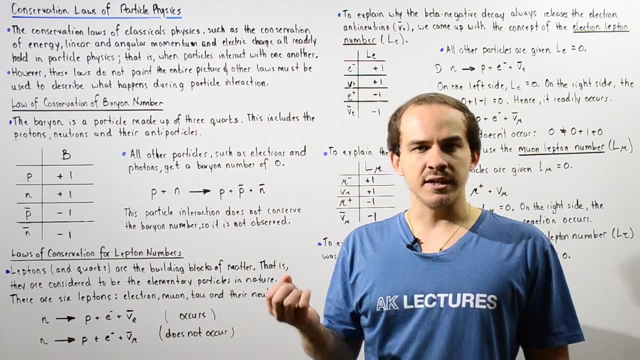 actually happens during particle interactions. So let's begin our discussion of the law of conservation of baryon number. So what exactly is a baryon? Well, a baryon is a type of particle that basically consists of three quarks. Now this includes protons, neutrons, as well as. 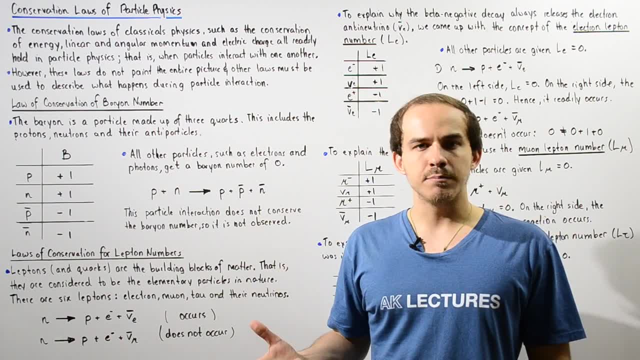 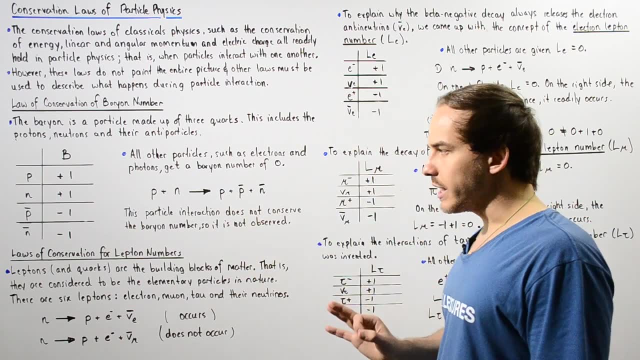 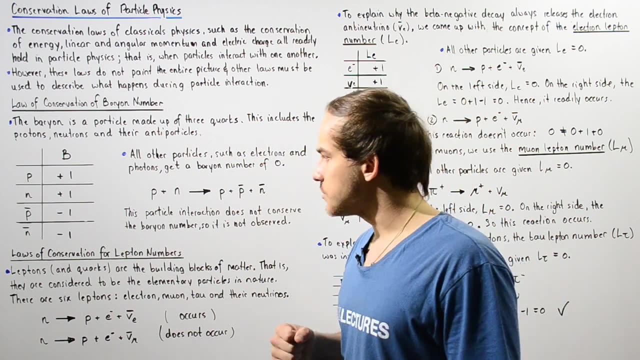 their corresponding antiparticles, the antiproton and the antineutron. So, according to this law of conservation, a proton and a neutron get a baryon number of positive one and their corresponding antiparticles, the antiproton and antineutron. 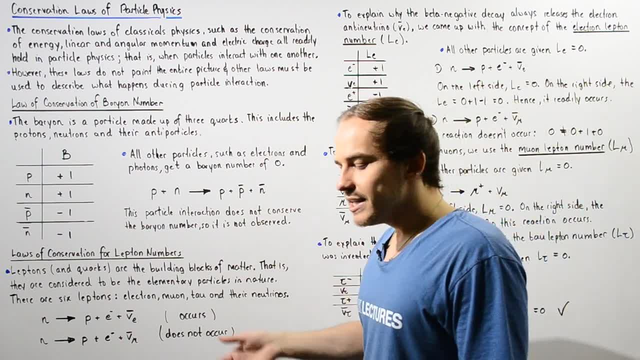 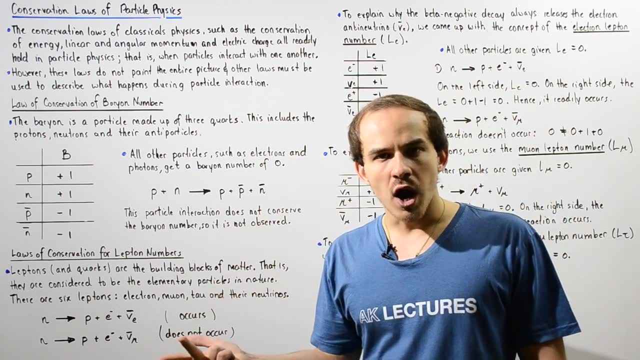 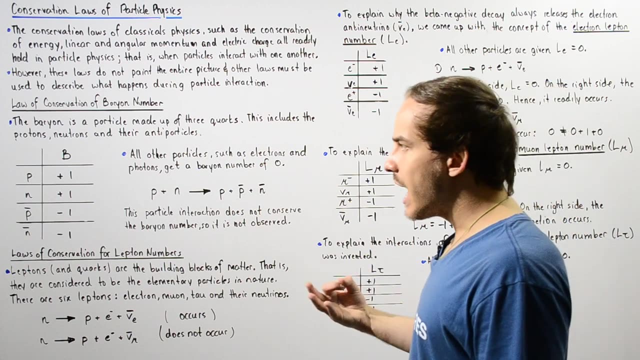 get a baryon number of negative one. Now, all other particles- and this includes particles such as photons, electrons, muons, neutrinos and other particles- get a baryon number of zero. So to see how this law of conservation of baryon number actually works, let's take a 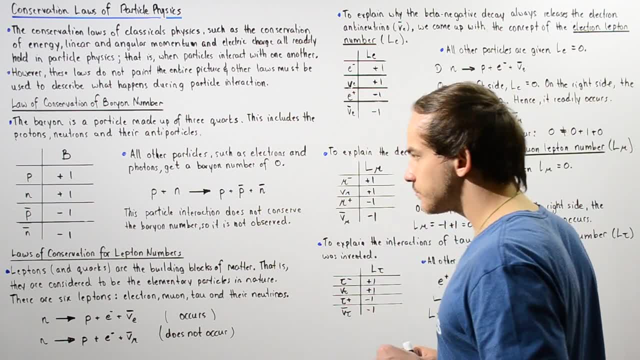 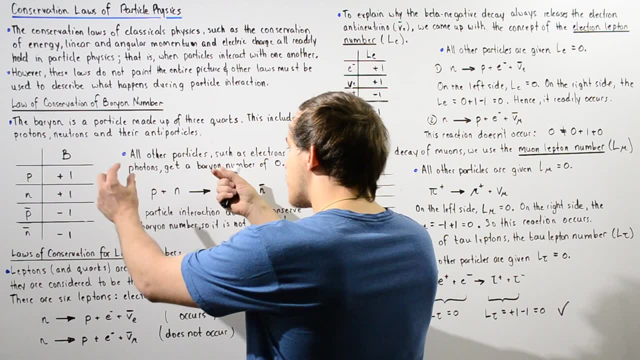 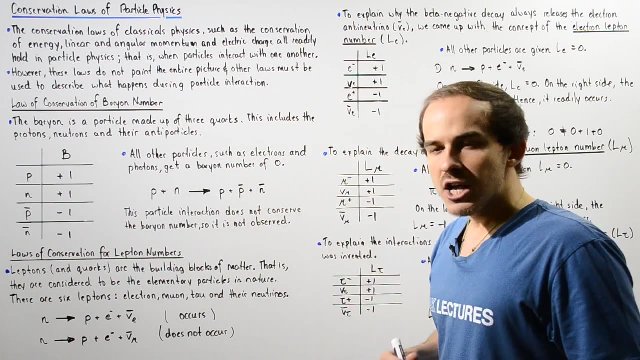 look at the following example. So let's suppose we have a proton that wants to interact with the neutron and during their interaction they produce a proton, an antiproton and our antineutron. So the question is: does this reaction actually occur in nature? Well, 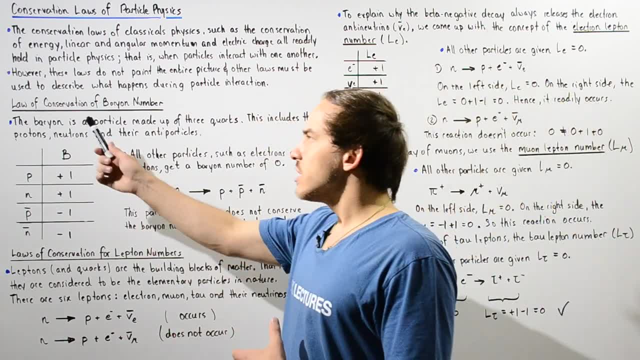 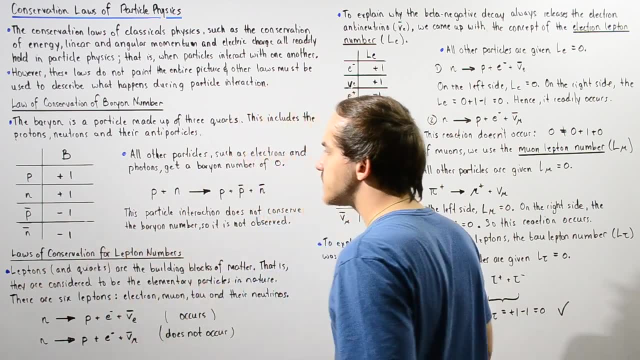 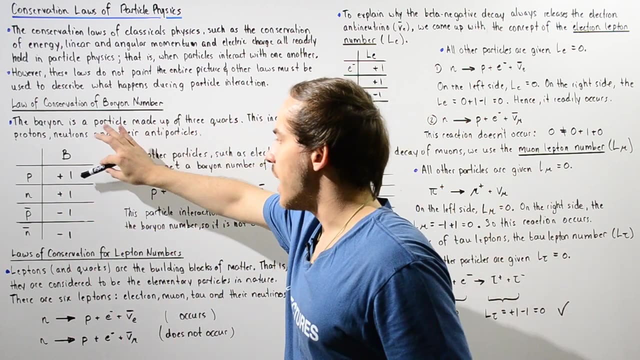 to see whether or not it occurs, we can use the law of conservation of baryon number. So, basically, let's calculate the baryon number. on the left side We have a proton-neutron, so the baryon number is positive two because each one has a positive one. However, let's 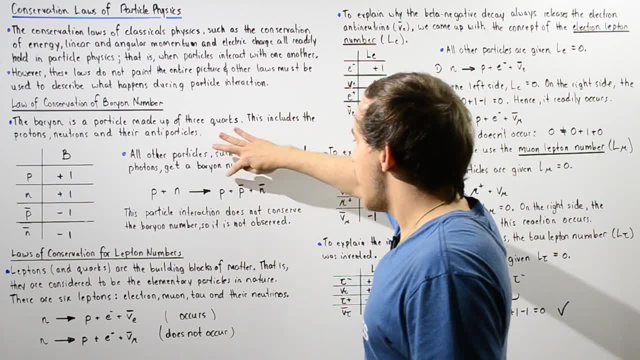 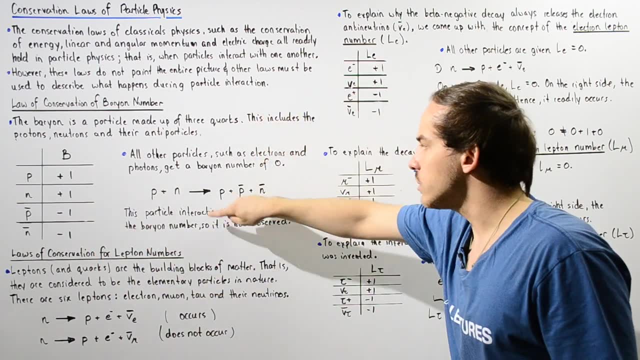 look, on the right side We have a proton, our antiproton and antineutron. So we have plus one minus one, minus one and the total number of protons, neutrons, neutrinos and neutrons And the total baryon number on the right side is negative. one Because positive. 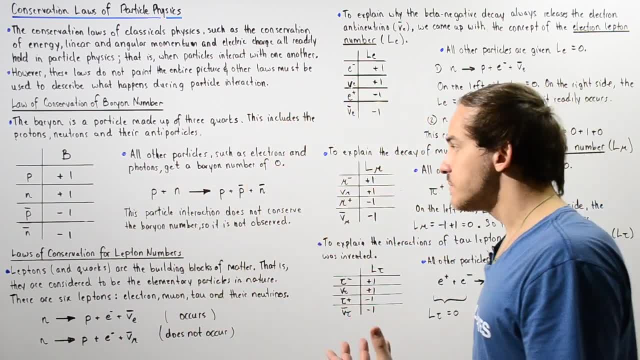 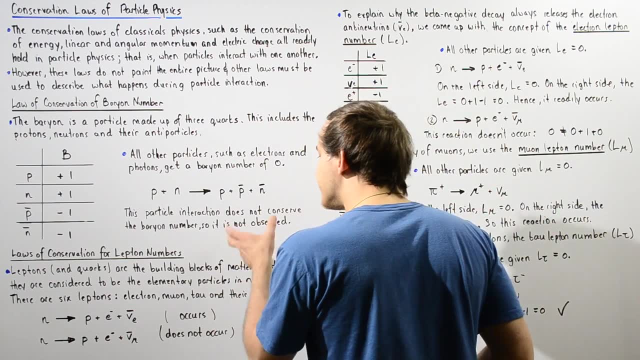 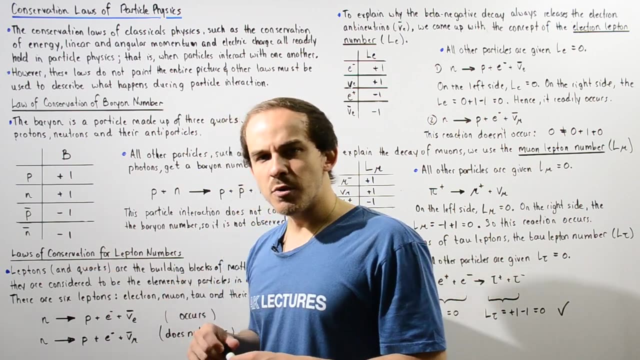 two is not equal to negative one. we see that this particle interaction does not actually conserve the baryon number, and so it will not take place in nature, And that's how we use the law of baryon number. Now let's move on to the laws of conservation for lepton numbers. There are three such laws. 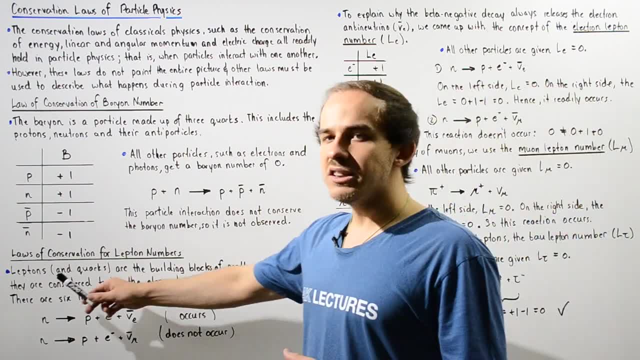 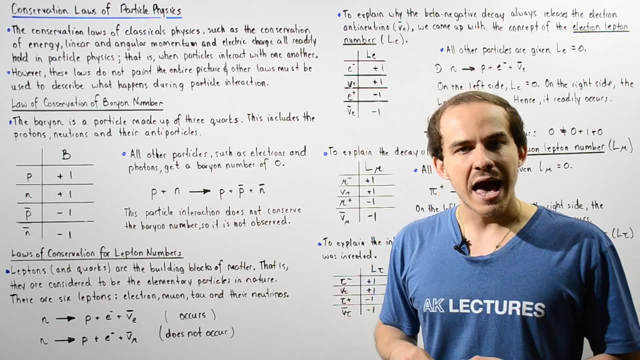 So one is the law of conservation of baryon number, and the other is the law of conservation of neutrons. What exactly is a lepton? Well, leptons, along with quarks, which are different from leptons, are the building blocks of matter. That is, these are the smallest type of particles. 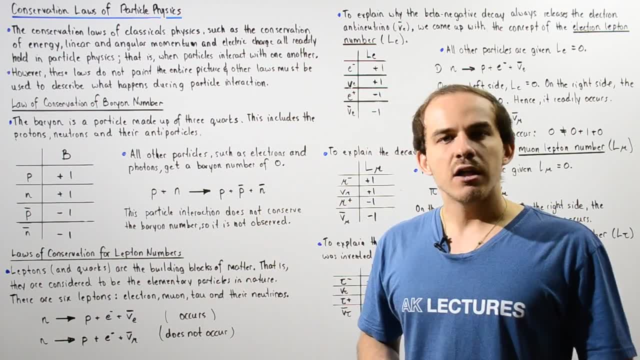 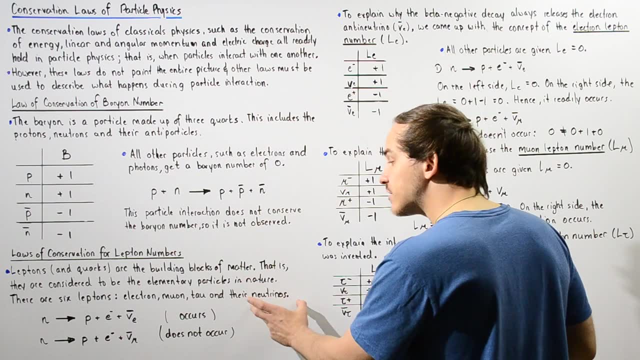 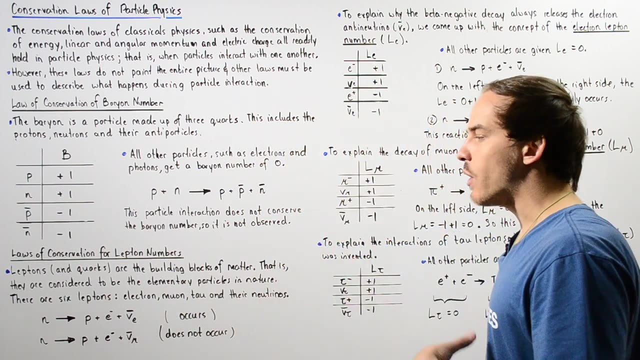 and they are known as elementary particles. Now, there are six leptons that we know of. We have the electron and the anta, or the electron neutrino. We have the muon and the muon neutrino And tau and the tau neutrino. as well as our anti-leptons, We have our anti-electron or 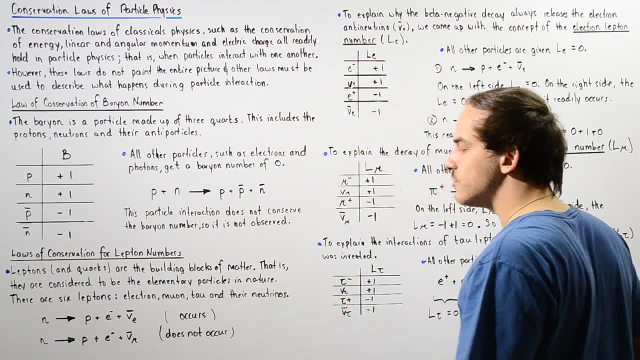 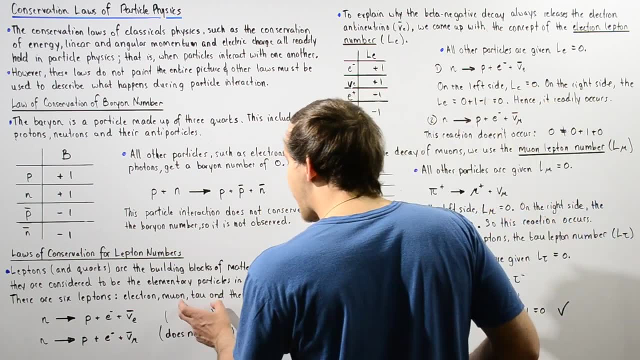 the positron as well as the electron anti-neutrino. We have our anti-muon as well as the muon anti-neutrino, And we have our anti-tau as well as the tau anti-neutrino. So basically, 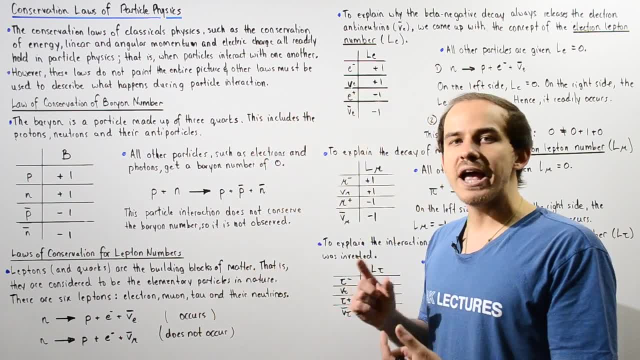 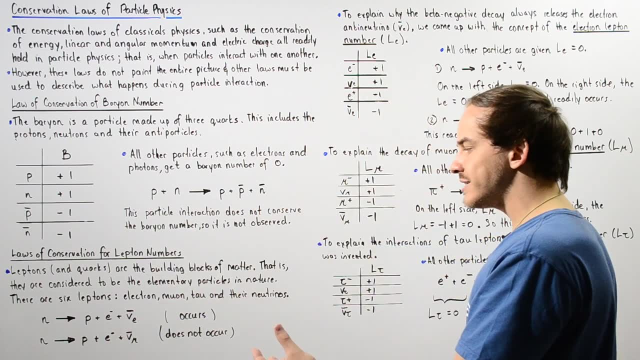 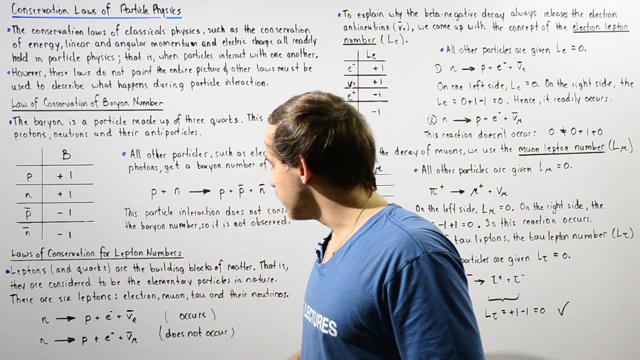 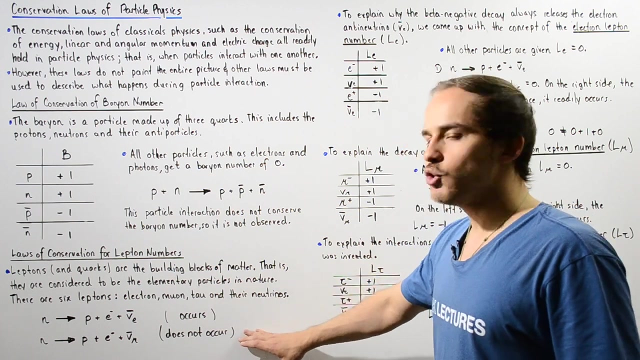 these laws were invented to describe the way that particles interact, specifically the way that electrons interact, the way that muons interact and the way that tau particles interact. So let's take a look at the following two reactions. So reaction 1 occurs in nature, but reaction 2 does not occur, So in 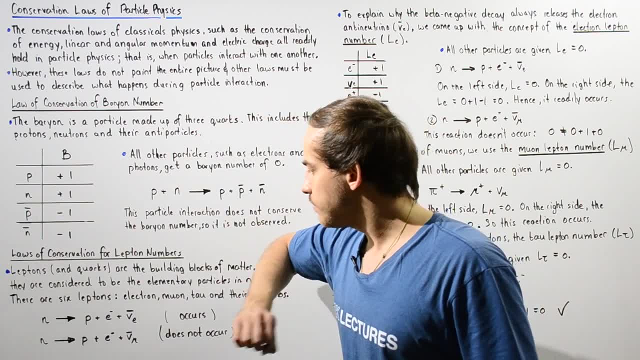 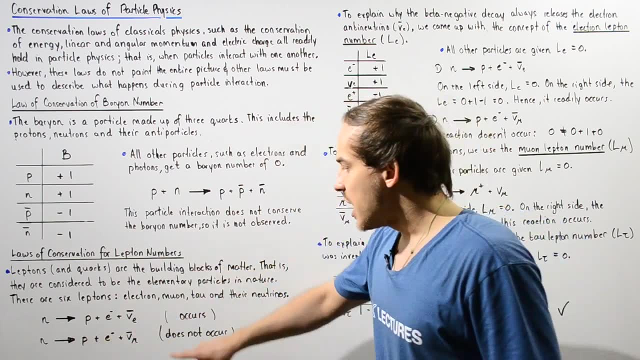 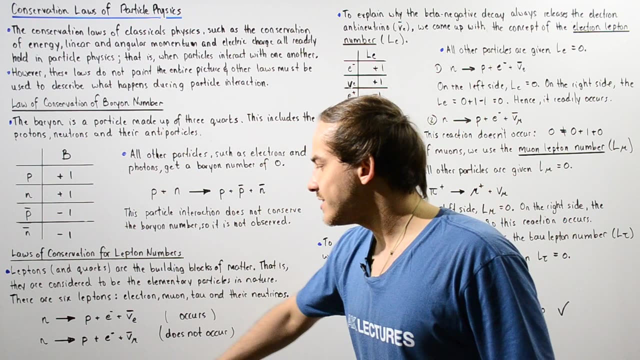 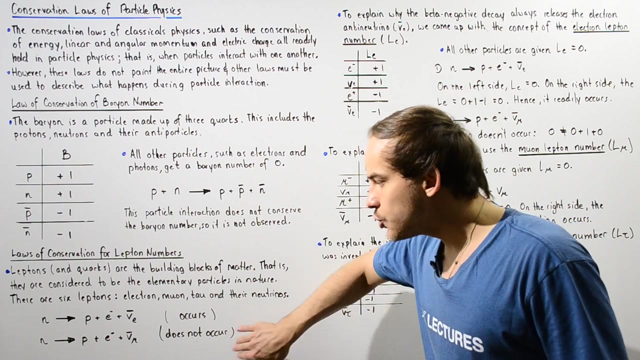 reaction 1: we have a beta decay taking place. We have that a neutron decays into a proton, an electron, as well as an electron anti-neutrino. Now the second reaction tells us that the neutron decays into a proton, an electron and a muon anti-neutrino. Now reaction two will never take. 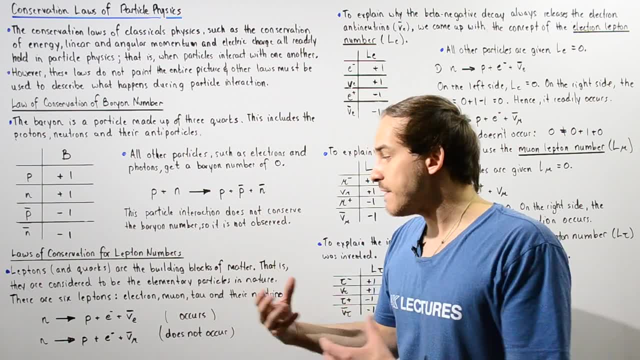 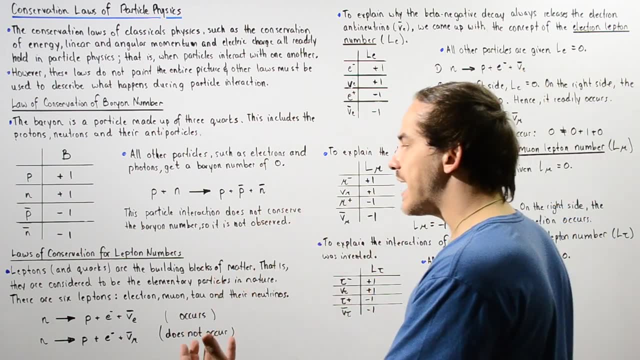 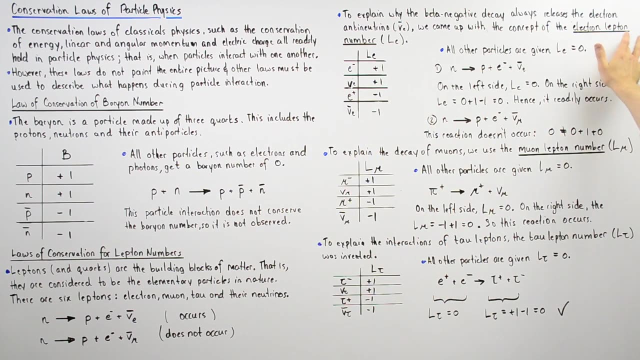 place And to explain or to describe the fact that this reaction does not take place in nature, we basically create the conservation of lepton numbers, specifically the law of conservation for electron lepton numbers. So to explain why beta negative decay always releases the electron, 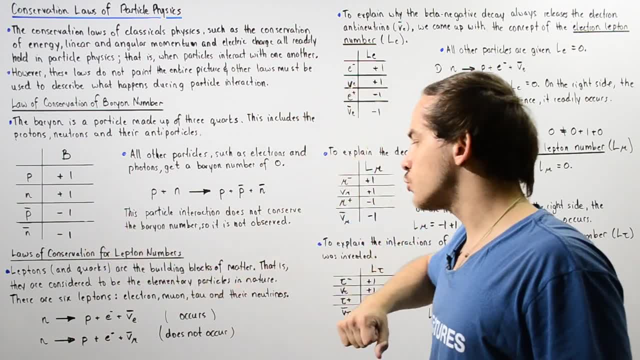 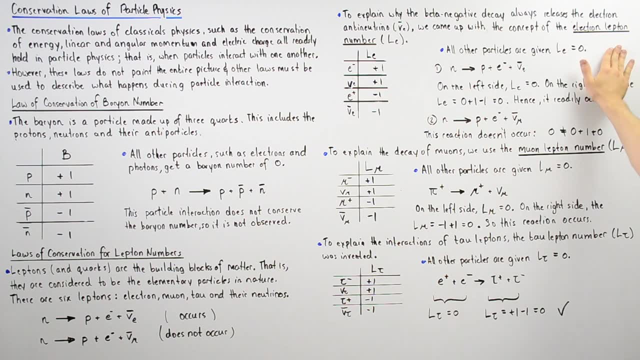 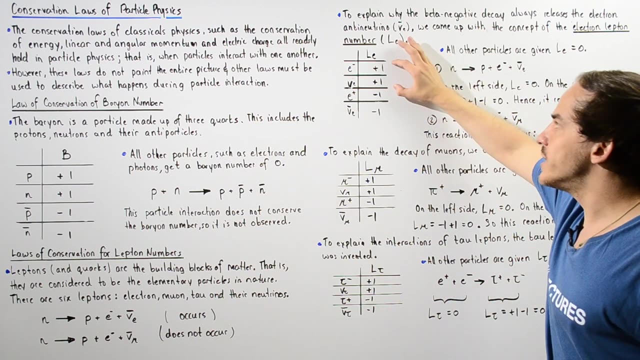 anti-neutrino and not the muon anti-neutrino or the tau anti-neutrino. we came up with the concept of the electron lepton number. So the electron lepton number basically tells us that if we're dealing with either the electron 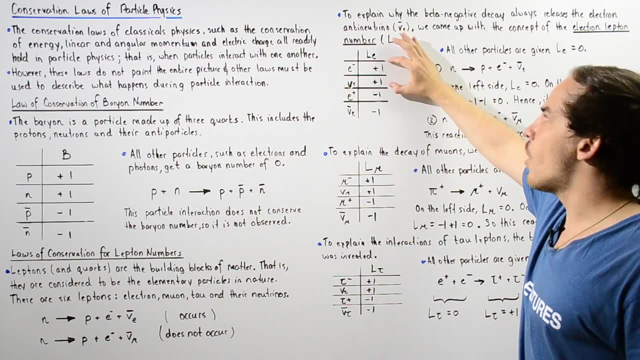 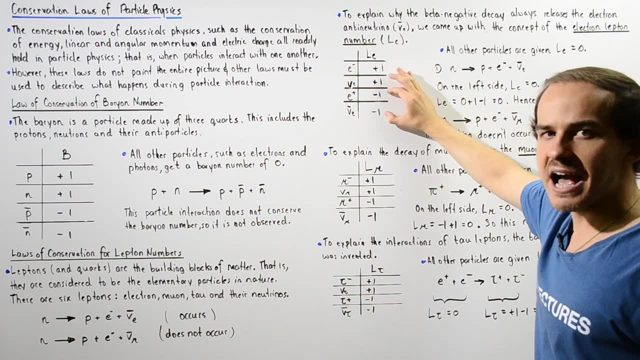 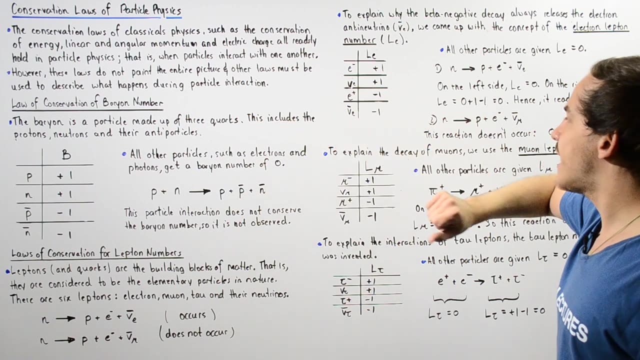 or the electron neutrino. these two particles get electron lepton number LE- of positive one, And their corresponding antiparticles, the anti-electron known as the positron and our electron anti-neutrino, get a value of negative one, And all of these particles get a value of negative one. 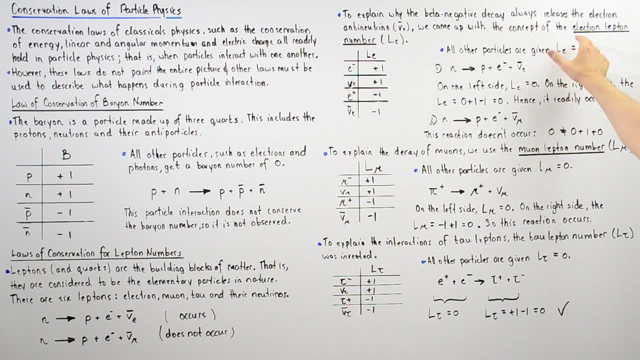 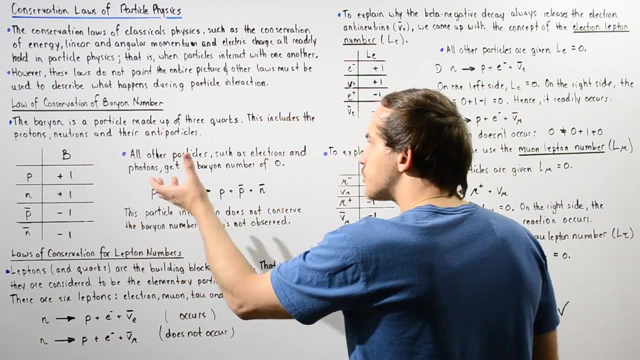 And all of these particles get a value of negative. one other particles get a value of zero for the electron lepton number. So in the same way that we had the conservation of variant number on the left and right side, we have to have the 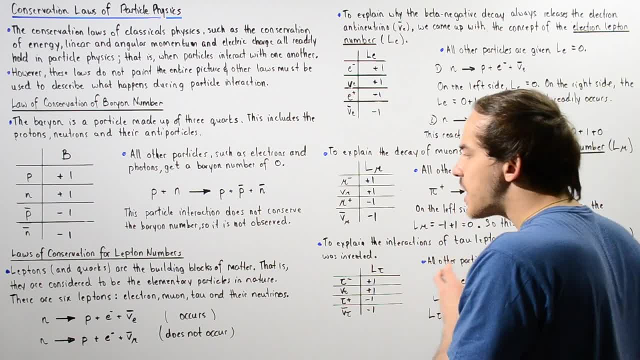 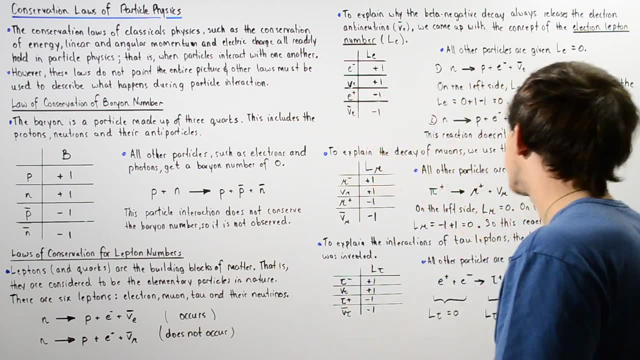 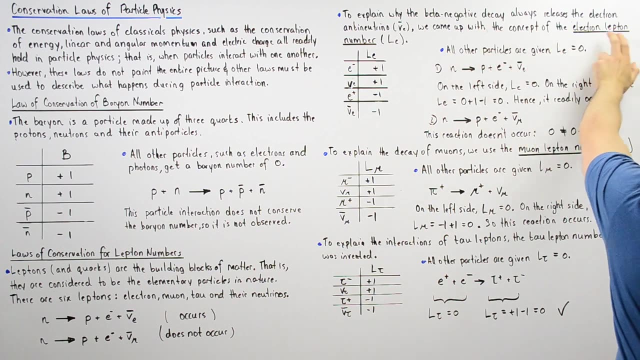 conservation of electron lepton number for that reaction to actually take place. So let's examine these two reactions. So why does reaction one take place? Well, on the left side of reaction one, we have a neutron and that gives and that gets an electron lepton number of zero. So on the left, 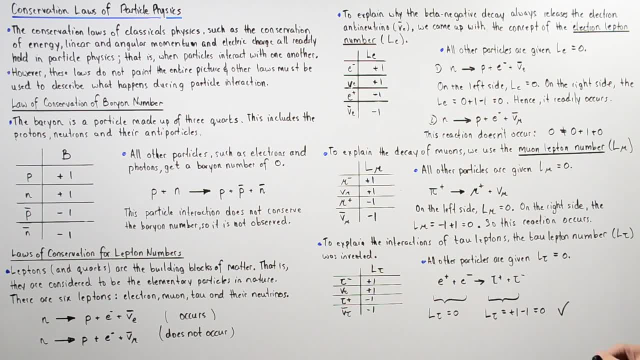 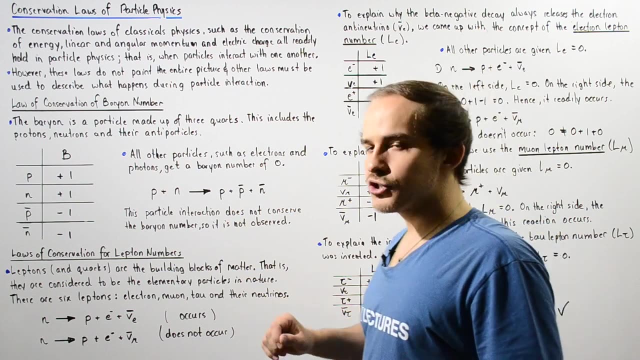 our lepton number, electron lepton number is zero. Now, on the right side, we have a zero, we have a positive one and we have a negative one, And this adds up to zero, because zero equals zero. This reaction takes place. What about reaction two? Well, reaction two on the left. 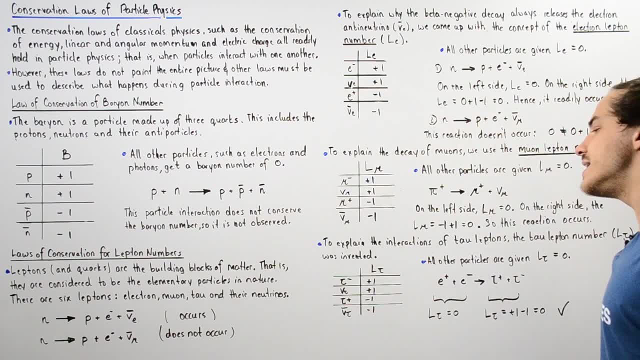 side we have a neutron, So it gives us a positive one. it doesn't equal zero. but on our right side we have zero. we have zero and positive one, And because zero does not equal positive one, this reaction does not take place. 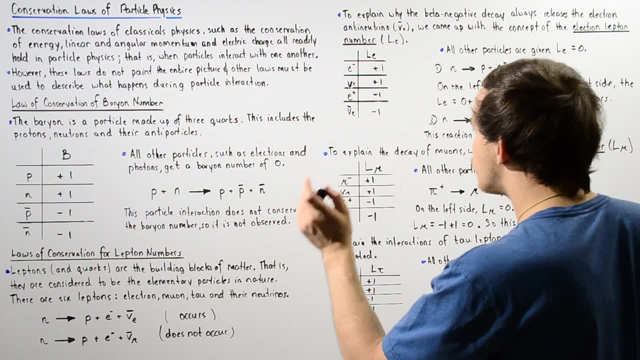 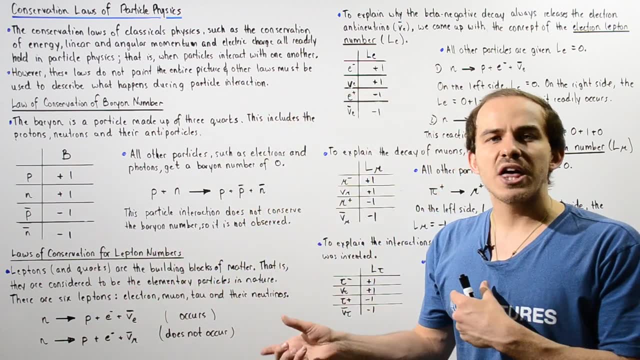 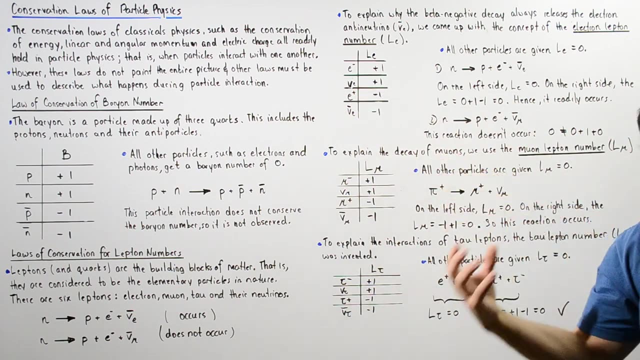 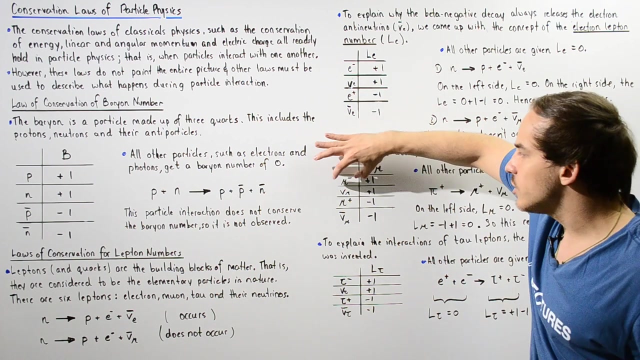 because it does not conserve our electron lepton number. So electron lepton numbers basically describe the way that electrons interact. What about muons? Well, to explain the decay or of muons, we use the muon lepton number given by L mu. Now, if we're dealing with the muon particle, 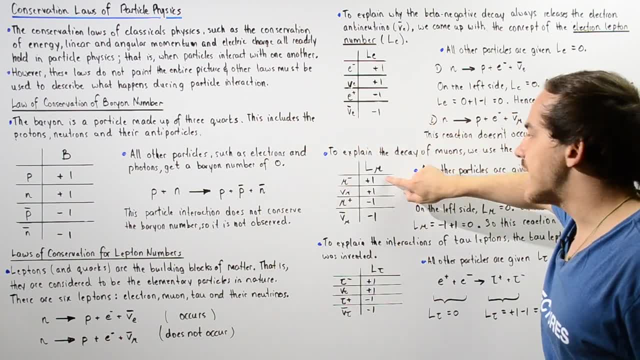 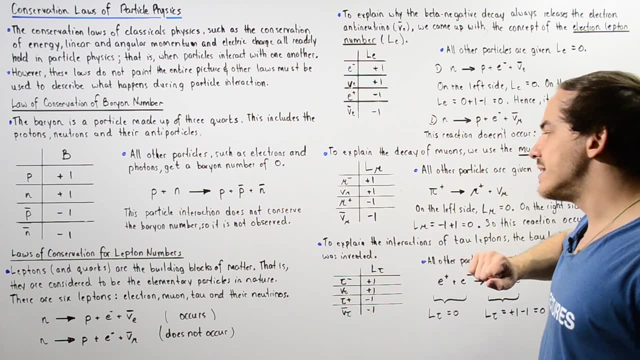 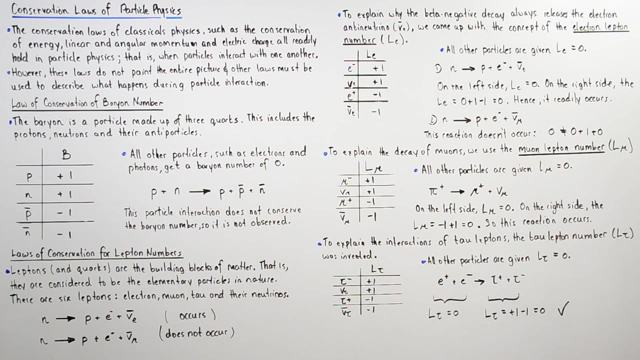 and the muon neutrino particle. these get a positive one. However, their corresponding antiparticles, the antimuon and the muon antineutrino, get a negative one. So all other particles are given a muon lepton number of zero. So let's take a look at this reaction. So on the 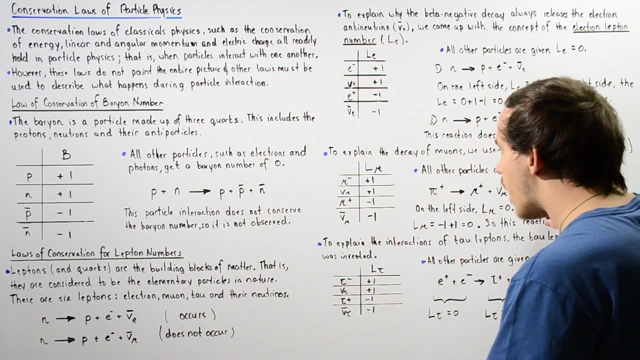 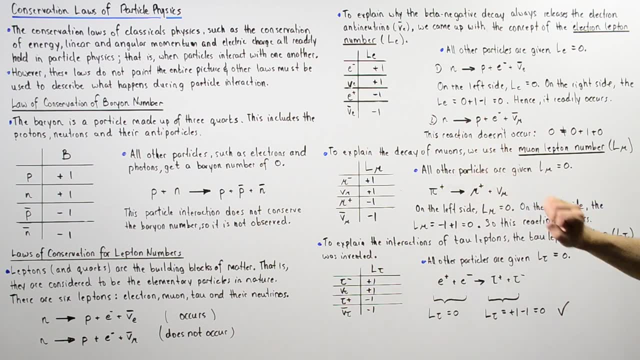 left side, we have something that is not a muon or a muon neutrino, so it gets a zero. On the right side, we have this plus this: This gets a negative one, this gets a positive one. so zero equals zero. 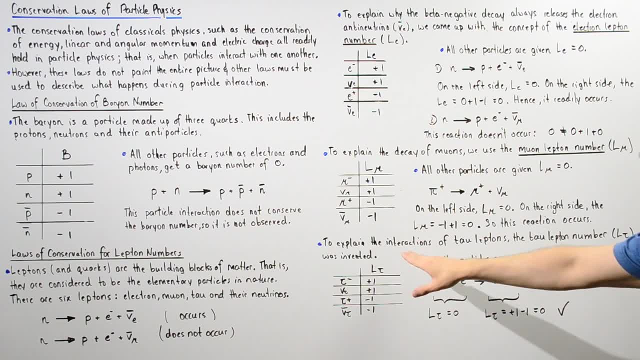 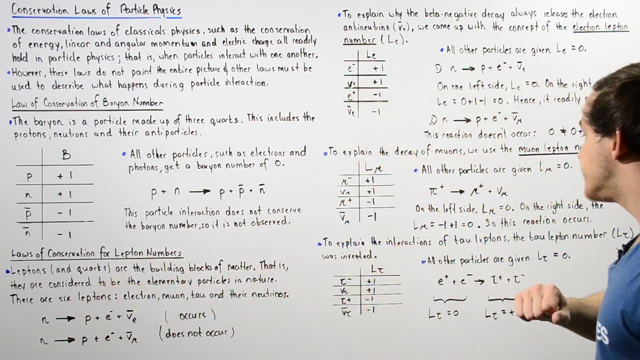 and that means this reaction takes place. And finally, to explain the way that our tau lepton interacts on the subatomic level, we came up with a muon lepton number of zero. So let's take a look at this reaction. So on the left side, 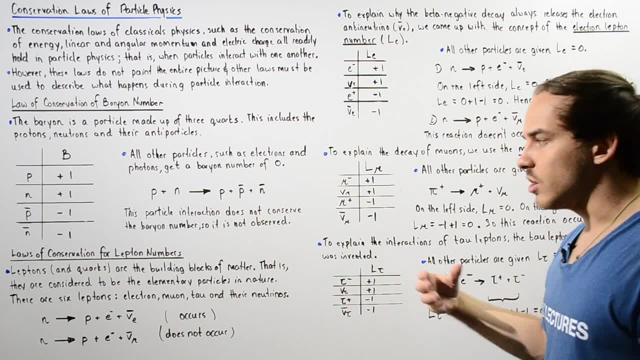 we have something that is not a muon or a muon antineutrino, so it gets a zero. On the right side we have something that is not a muon or a muon lepton number of zero. So basically, this is the. 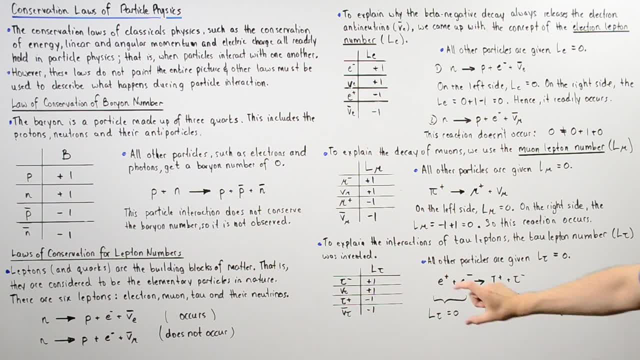 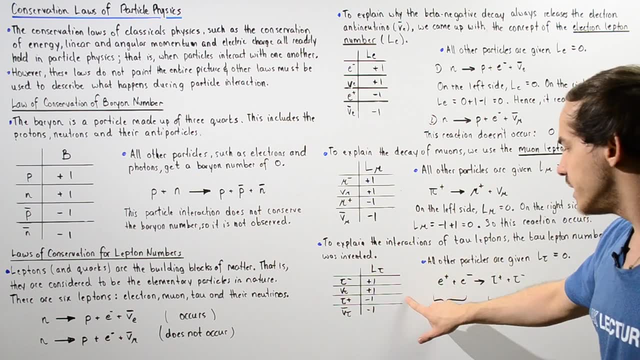 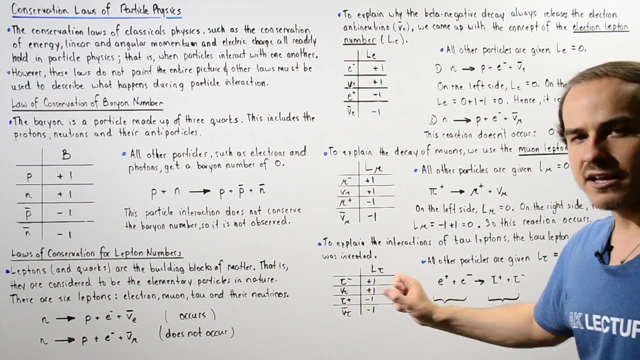 law of conservation of tau lepton number. So once again we see that tau and its corresponding neutrino, tau neutrino, get a positive one and their corresponding antiparticles, the antitau and the tau antitrino, get a negative one. So let's look at this reaction. We have the electron. 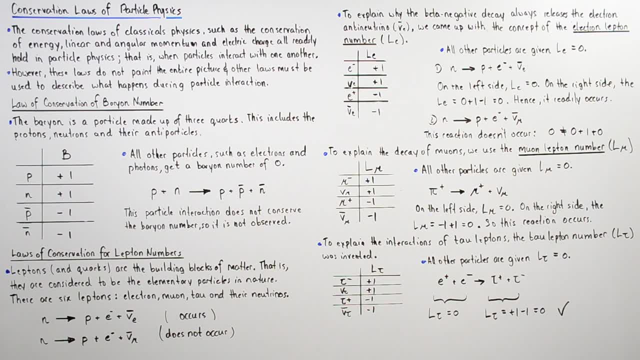 combines with our positron and that releases the lepton number of zero. So on the right side, our tau and anti-tau. Now tau and anti-tau sum up to zero. We have positive, negative one and these both get zero, Because zero equals zero. we see that our law of conservation of